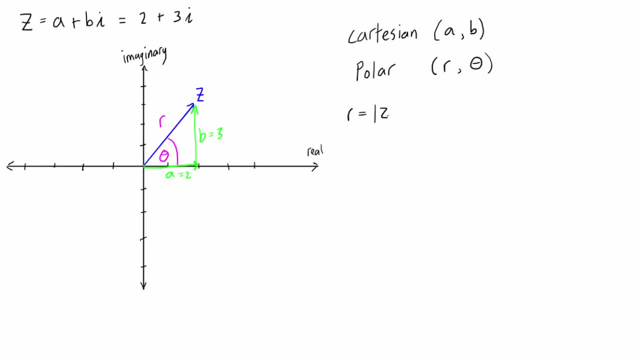 because r is just equal to the modulus of z, Which was equal to the square root of A squared plus B squared. And again, if you look at this geometrically or thinking about this as a triangle, it's basically Pythagorean theorem where A squared plus B squared equals C squared. 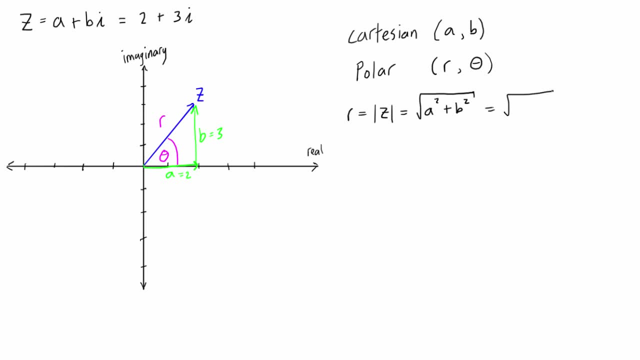 So if we just fill this in a little bit, we get the square root of 2 squared plus 3 squared, which is the square root of 4 plus 9, which is the square root of 13.. So this is the modulus of z and this is also. 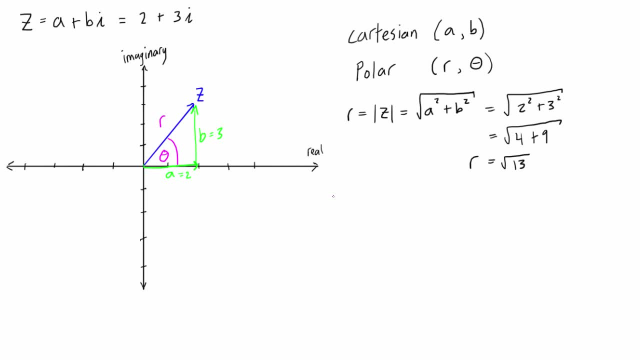 our value for r when we're looking at it in polar form. And theta is pretty easy to get as well, because the tan of theta is just equal to B over A Right. it's the opposite over the adjacent side. And we can just rearrange this and say that the tan inverse of 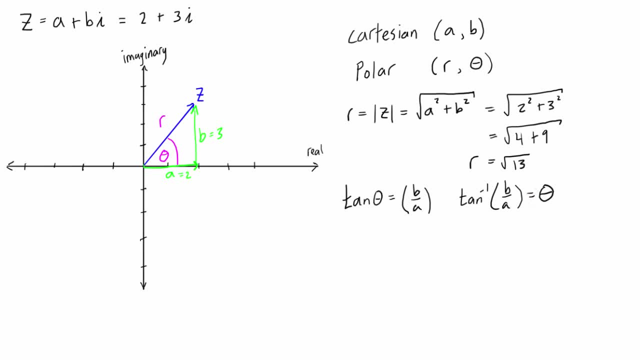 B over A is going to give us theta And if you remember, when we're dealing with polar coordinates we should be using radians. Theta we call the argument of z- Sometimes you'll be hearing that- And if theta is between negative pi to positive pi, 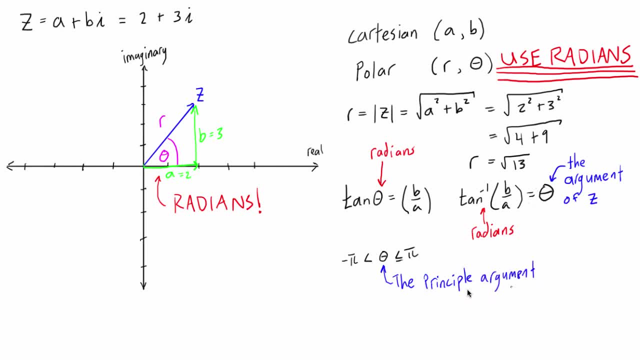 we call it the principal argument And the reason we make this distinction here for the principal argument is because there's actually an infinite number of thetas that work for defining this complex number in polar form. Because we have, if we imagine that we start rotating our angle here from the real axis. 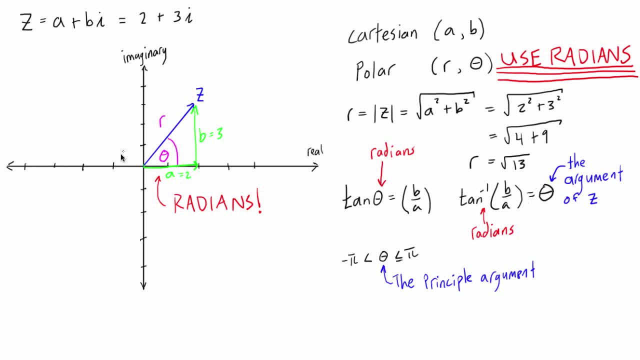 we can come out to theta. But if we add another full rotation, which is 2 pi radians, we're going to have a different theta. It'll be basically with this theta, this angle plus 2 pi, And then- and that satisfies our format here- 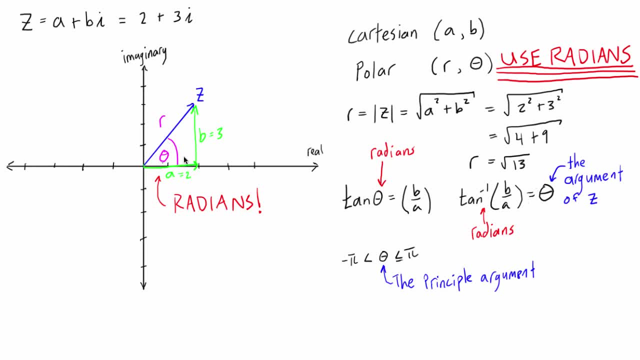 We can add another 2 pi. we can add another 2 pi, or we can subtract basically any integer multiplier of 2 pi's, And so, basically, the simplest theta that we can deal with is one that is basically in this first half of the rotation, or 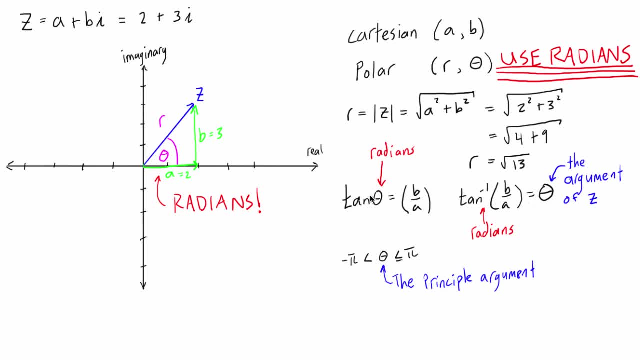 in this area, And so that's basically the simplest theta that we can deal with is one that is basically in this first half of the rotation or in this area. So if you're using your calculator like this with tan inverse function, it will spit out a value and you just have to check by. basically, I would recommend plotting the. 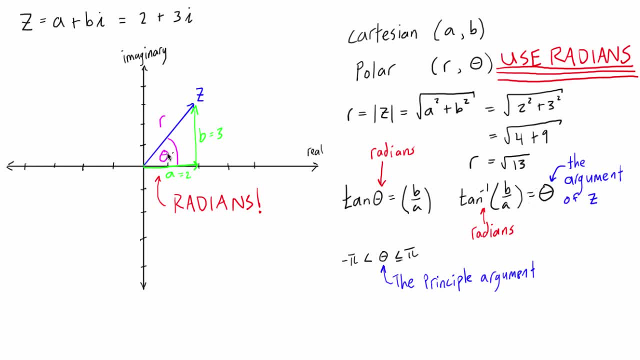 vector here, as you can, using a and b in the Cartesian point and just identifying which quadrant it is- Is it 1,, 2,, 3, or 4?? And I would just double check that the value that you're getting for your theta here actually reflects that you're in the right. 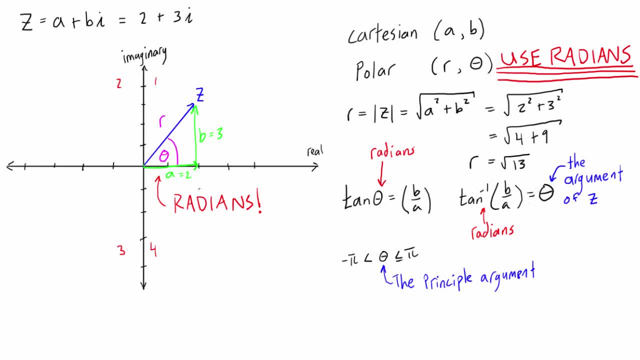 quadrant and not the one that's like diagonally across from it, Because that is possible using your calculator. If that does happen, then you just have to subtract pi from it to get the proper theta that we're looking for. Okay, so now what we want to do is we want to actually just write the complex number in polar form. 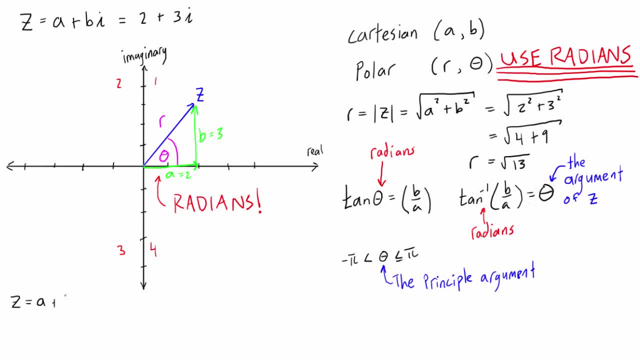 So if we start with the form, z is equal to a plus b i. we can convert this from a's and b's to r's and thetas. So if we look down here, a, a is equal to r cos theta and b is equal to r sine theta. 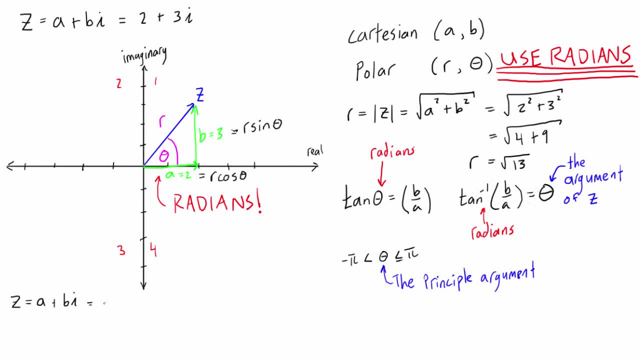 So we can make this substitution here. So we have: this is equal to a, so a is r cos theta and plus b i, so b is r sine theta times i- and it's actually nicer to write the i out front- r sine theta. 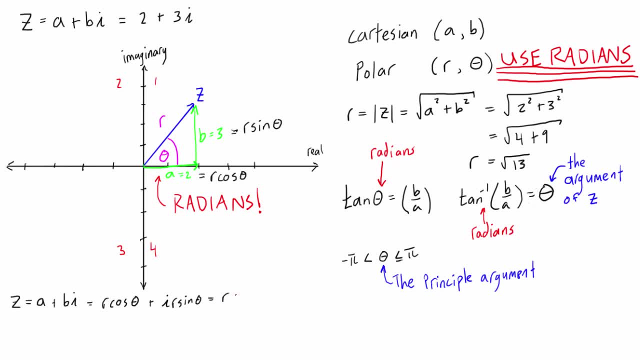 What we can do is we can pull out the r, because it's common to both terms. So we have r times cos theta plus i sine theta, and now we have it all in terms of r's and thetas, And sometimes you might also see it written like this: where we have the 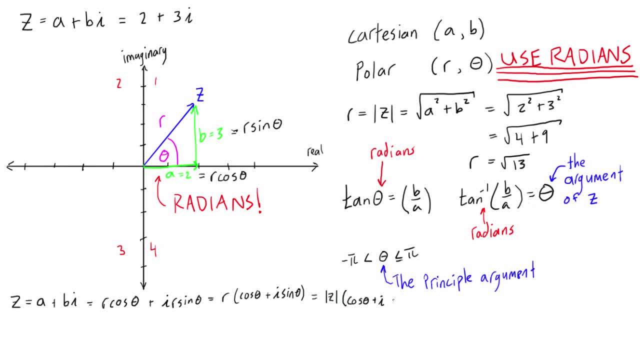 modulus times cos theta plus i sine theta, But whether or not we use r or modulus, basically when we have modulus, times cos theta plus i sine theta, or r times cos theta plus i sine theta, now we have converted it into polar form. 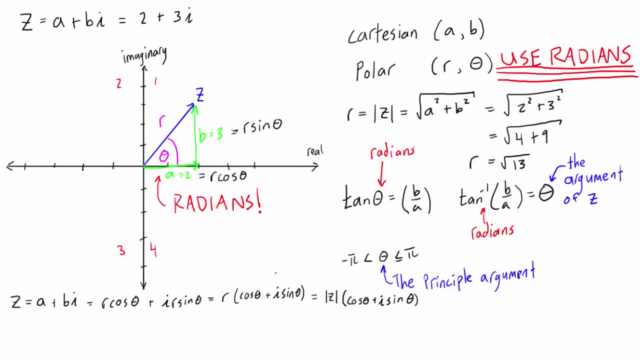 So let's actually write what we have here for our numbers. We need to figure out what theta was, and so theta is equal, and we can continue over here. theta is equal to tan inverse of b over a, so the tan inverse of b over a, so b is 3. 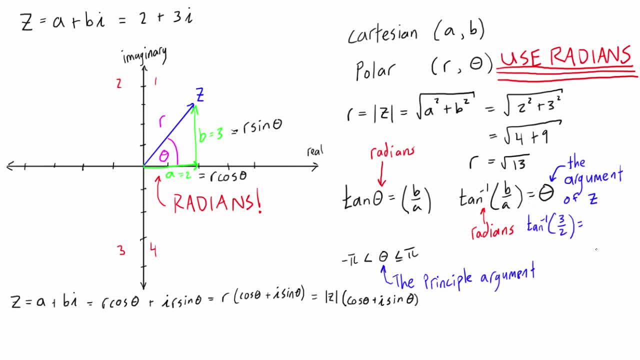 over 2.. If we put this in the calculator with radians on, we find this is 0.983, and the decimals go on forever. but let's just cap it at 3 here for now. So this is equal to theta.